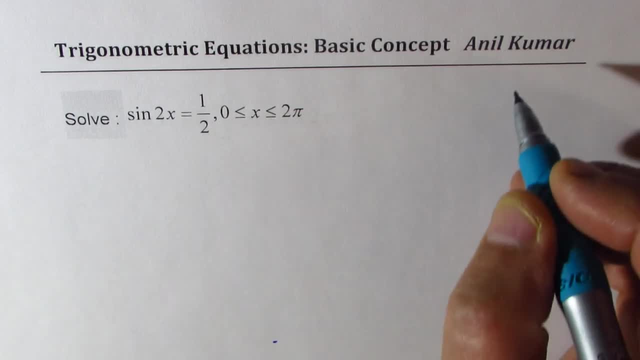 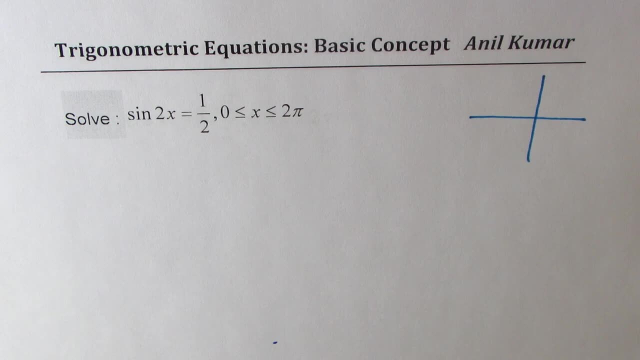 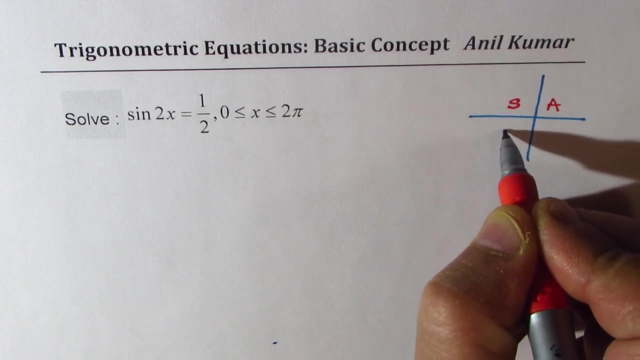 Now what you need to remember here is a few basic things. We're looking for sine to be positive. That means we're looking for solutions in two quadrants. Correct, You know, all are positive in quadrant one. Sine is positive in quadrant two, Tan is positive in quadrant three And cosine is positive in quadrant four. 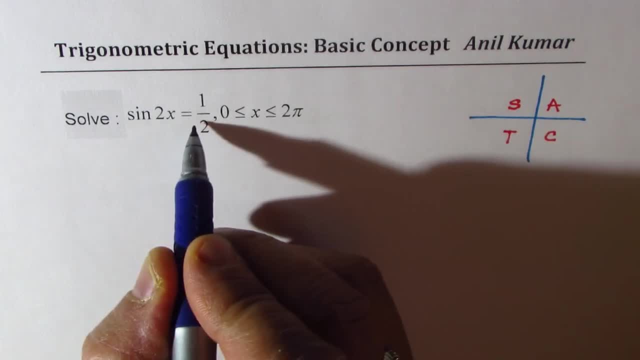 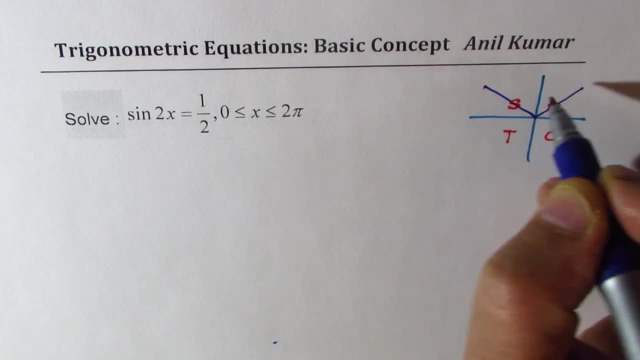 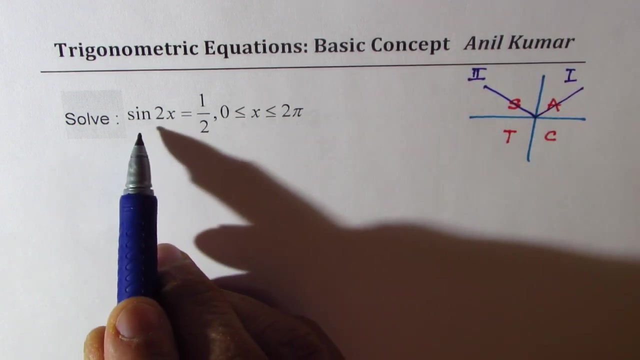 So when we are given that sin 2x is positive, we mean we have two solutions, right? So we have these two solutions. We have solution in quadrant 1 and also in quadrant 2.. In both the quadrants, sin is positive. That is one thing which you should know, right? So this: 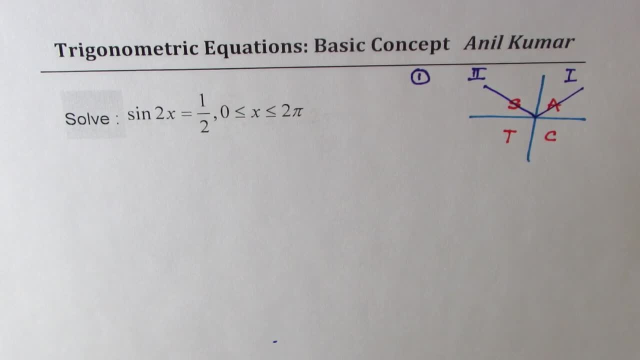 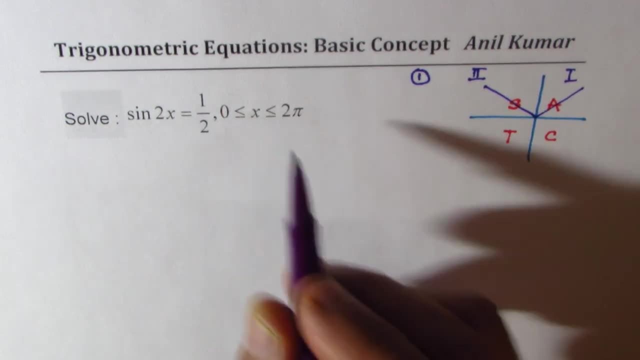 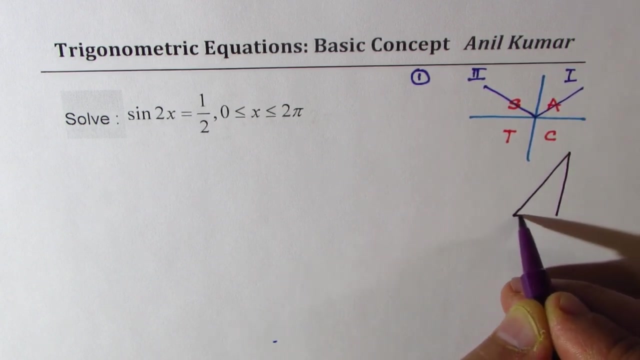 is first thing which you should know. Second, when we are looking for values like 1 over 2, that reminds us of a special triangle, right? So I will sketch the special triangle here for you. Whenever you are solving trigonometric equations, keep in mind these special triangles. 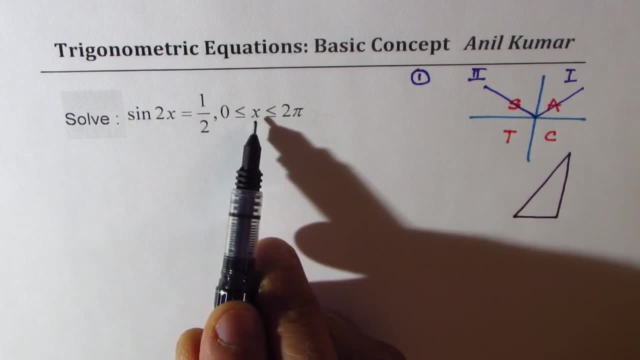 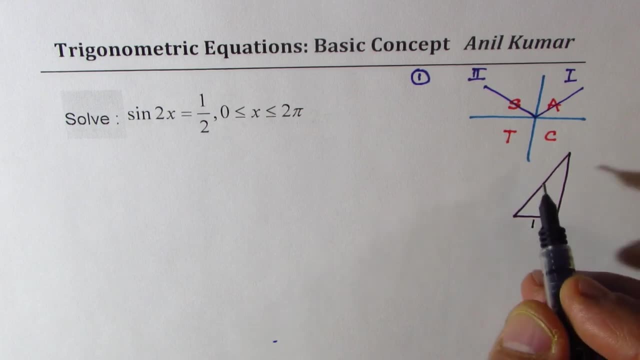 We will work with radian, since domain for x is 0 to 2 pi. Now when is sin half? So this triangle is 30,, 60,, 90, or in radians. what do we say? This is pi by 3,, this is pi by 6 and that is 90, right? So that is the triangle of. 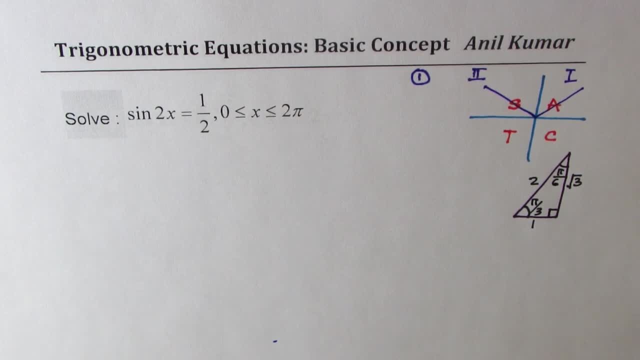 our interest, Perfect. So this is the second thing which you should know. Third, this is the triangle of our interest. So this is the second thing which you should know. Third, this is the triangle of our interest. Third, this is the triangle of our interest. So, 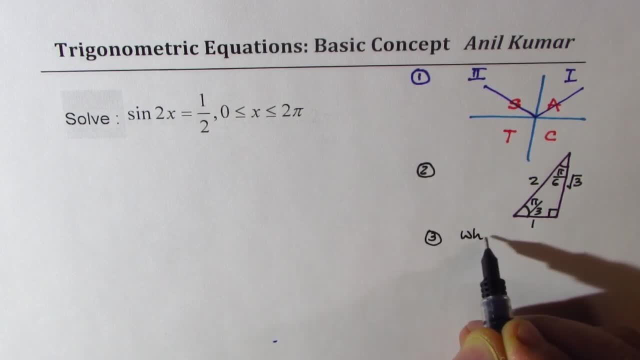 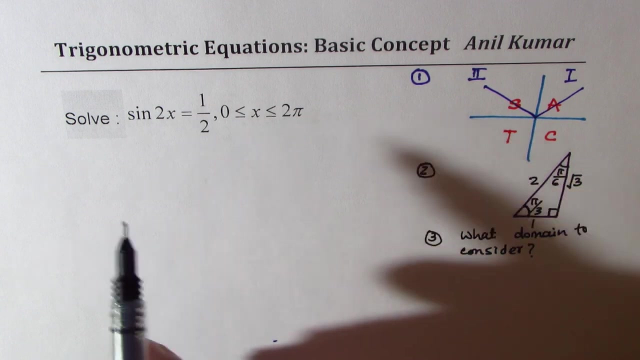 this is the triangle of our interest. So, this is the triangle of our interest. Now, the third thing which you should know is what domain to work on. Well, of course, we are given x is from 0 to 2 pi, but remember, this is sin 2 x, So that makes it very tricky. 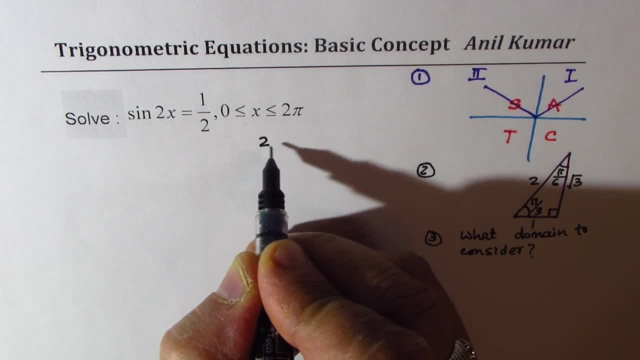 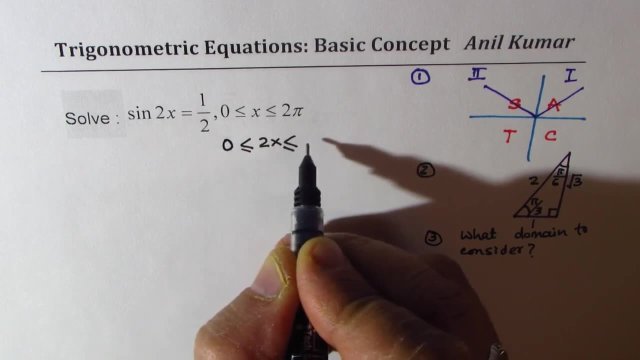 So x is between 0 and 2 pi. How about 2 x? 2 x should be between sin 2 and sin 2.. So we have to multiply these by 2.. So we get a modified domain for 2x and which is between 0 to. 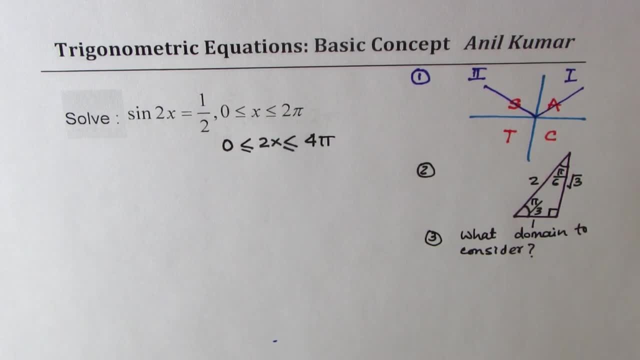 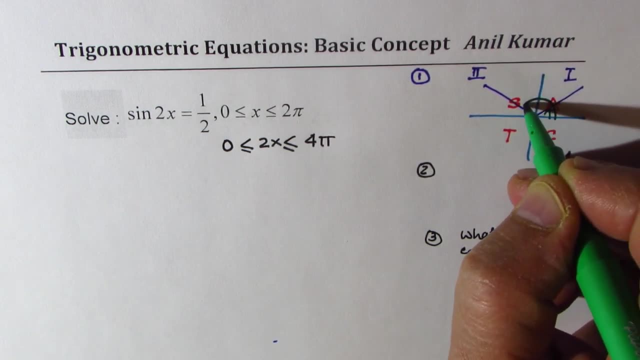 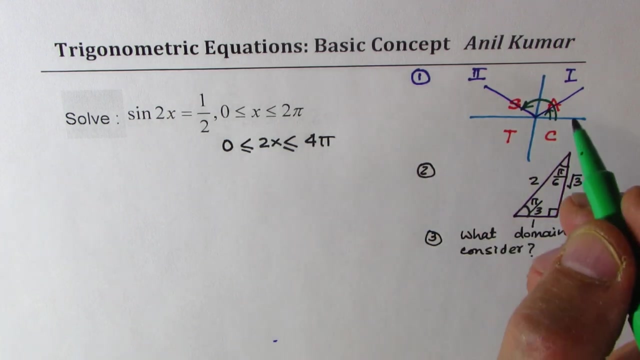 4 pi, You get the idea. So 0 to 4 pi really means this is our first solution. that is the second solution, correct? These are the two solutions within 0 to 2 pi. Now, when we consider 4 pi, 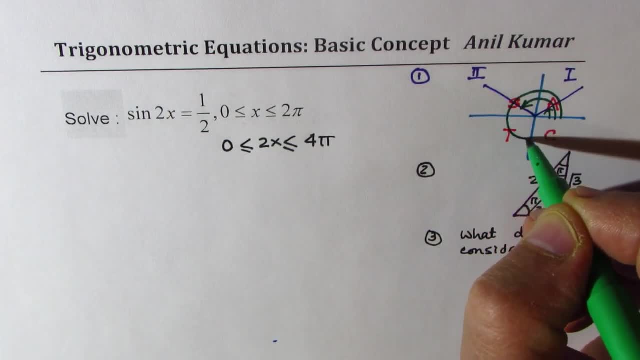 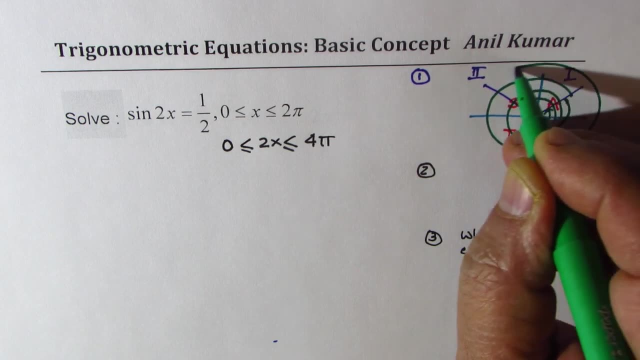 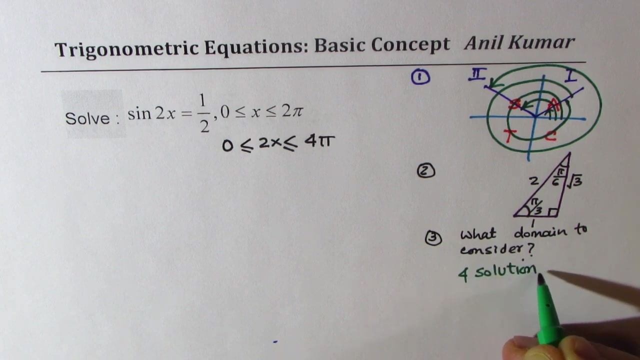 that means we are considering the solution which is one circle here and then also which is this circle, So we are expecting four solutions. Do you get that part? So if you miss the later two solutions, you have only done half of the question right. You may not even get half the marks. That is important to understand. 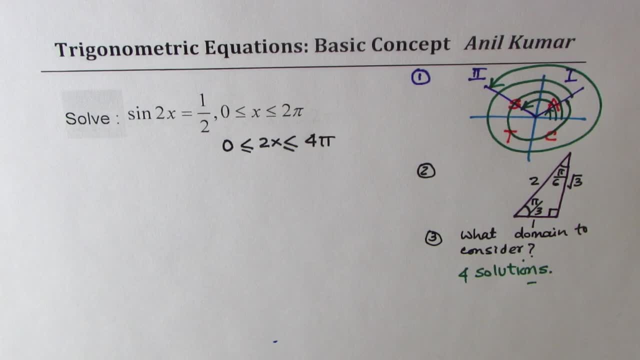 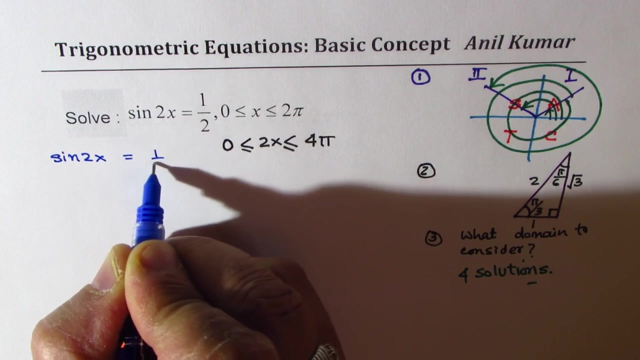 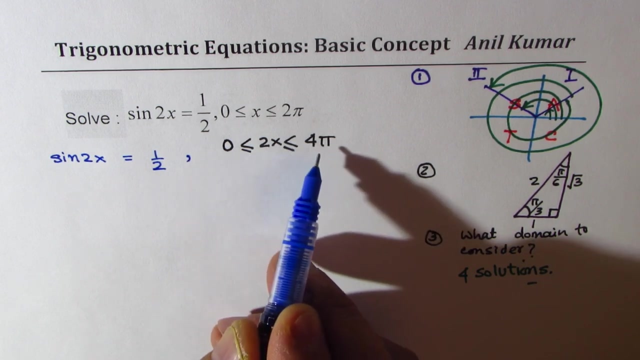 So I hope all the concepts are now clear and let us see how to solve this question right. So let us begin with the equation given to us, which is: sin 2x equals to half. As soon as you see this, you should modify the domain. So 2x is between 0 and 4 pi. Now, when 2x is between 0 to. 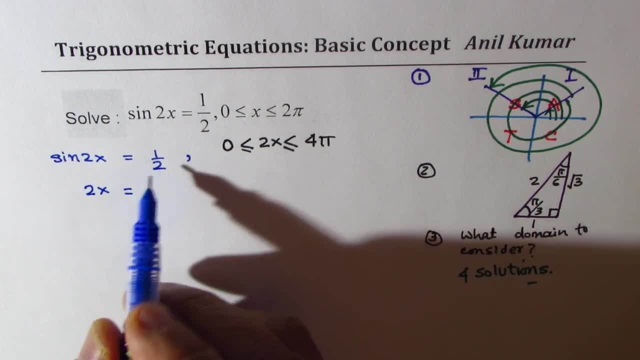 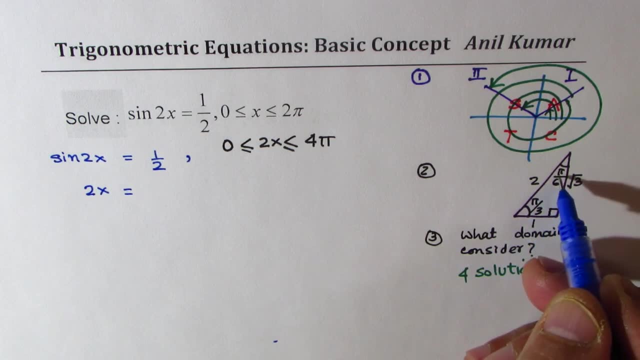 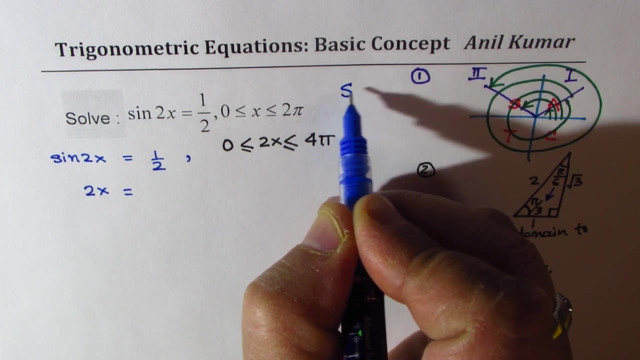 4 pi. what are the possible values of 2x for sin, 2x to be half. Now, clearly, from here, sin is half when you are looking from pi by 6, right? So that is the opposite side. We know sin is opposite. 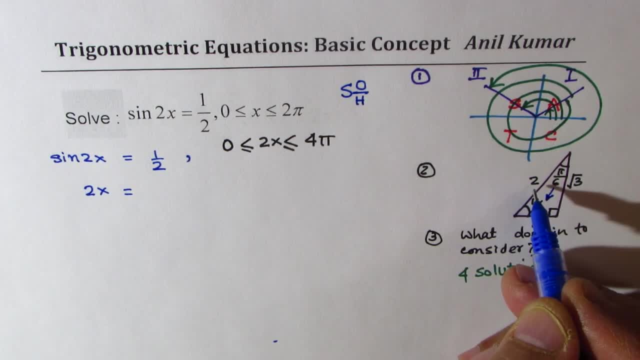 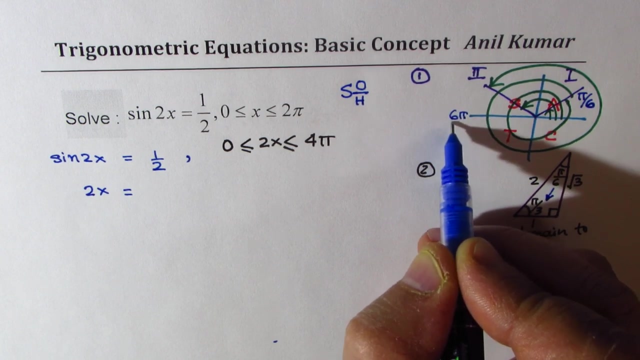 over hypotenuse, correct. So 1 over 2.. So the angle is pi by 6.. So this angle here is pi by 6, correct? The other angle in this quadrant will be now: pi is 6, pi by 6. Think like this, So that one is 5 pi. 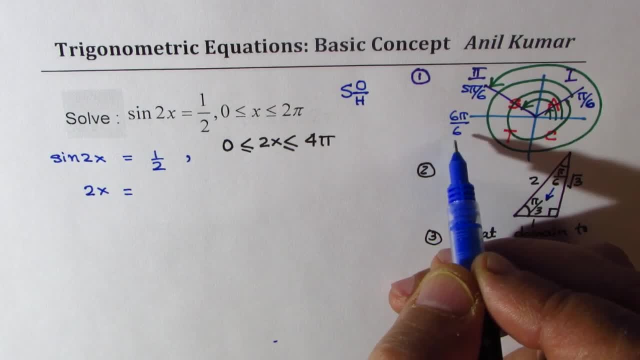 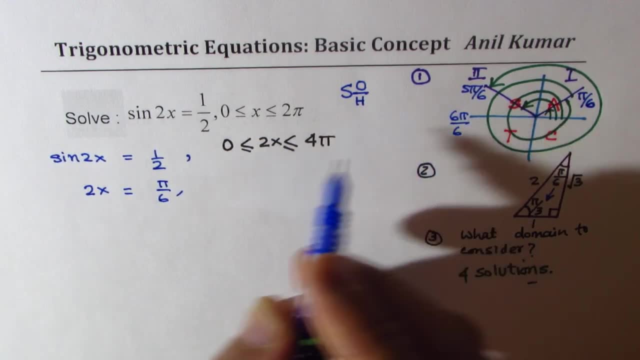 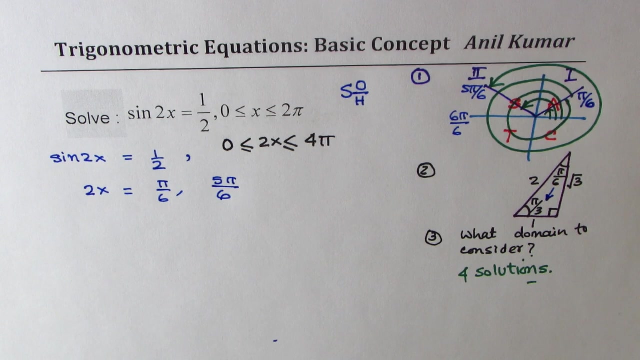 by 6, correct One less than 6, pi by 6.. So that is, we get the first two solution, which is pi by 6, and we also get 5, pi by 6.. Now we need to get two more. How are you going to get two more? 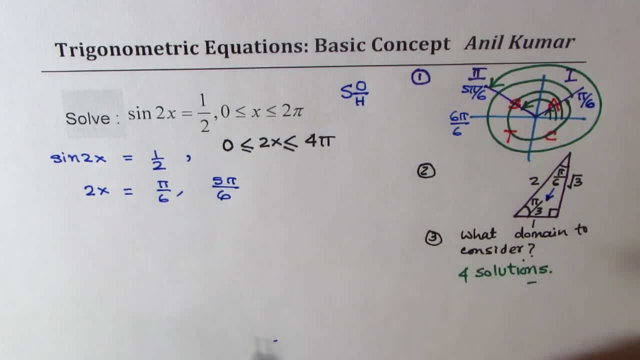 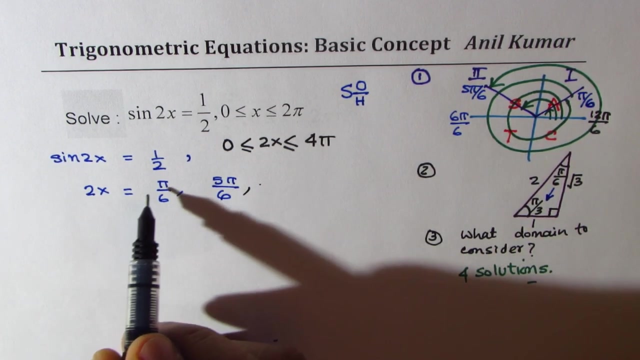 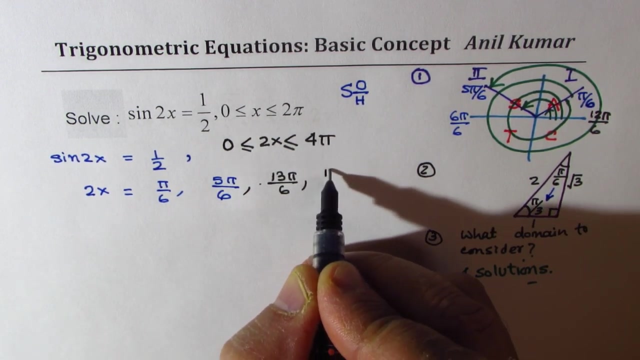 We have to add 2 pi to this. right, We have to add 2 pi. Easy way to add 2 pi is in terms of fraction of 6 as 12 pi by 6.. So if I add 12 pi by 6, I get the other two. 12 plus 1 is 13.. So we get 13 pi by 6, and 12 plus 5 is 17.. 17 pi. 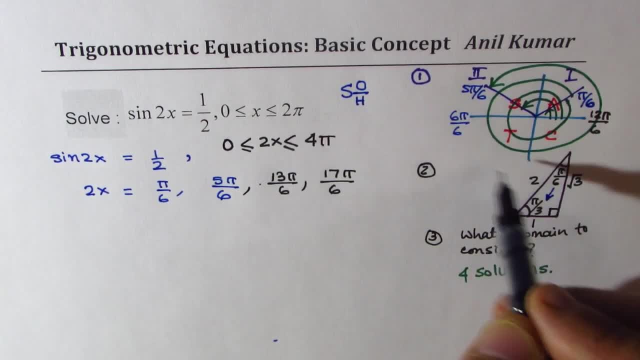 by 6. Do you get this part? So for the second circle we added 2 pi. 2 pi is equal to 12 pi by 6.. Do you see that? It's like 2 pi by 1. Multiply by 2. You get 12 pi by. 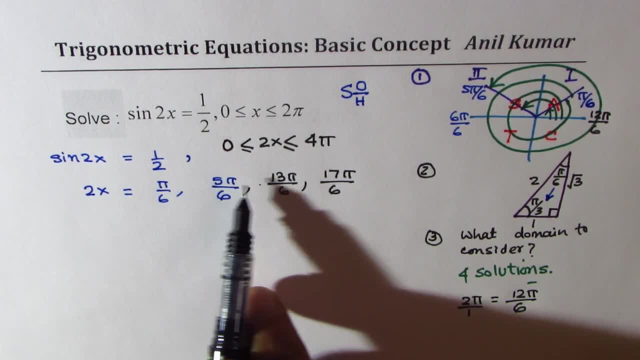 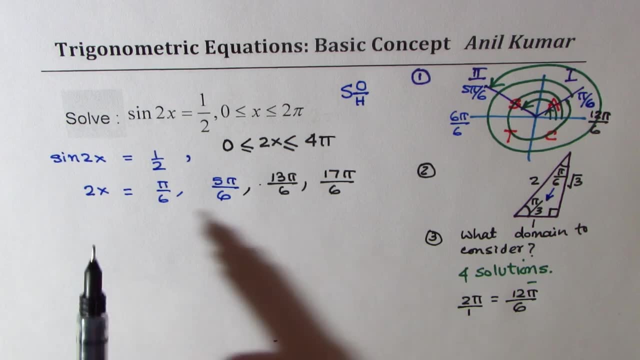 6.. Now it's easy. Just add 12 to the numerator. What denominator of 6?? So you get possible values of 2x, right? So don't leave the question here. The actual answer is to find x, So we'll go one. 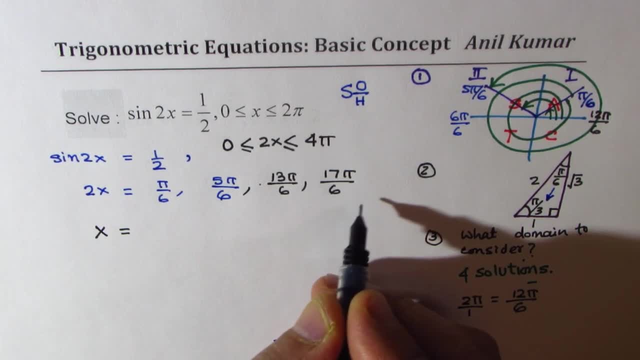 more step, and so x's divide these by 2pi by 6.. So we'll go one more step, and so x's divide these by 2pi by 6.. So we'll go one more step, and so x's divide these by 2pi by 6.. So we'll go one more step. 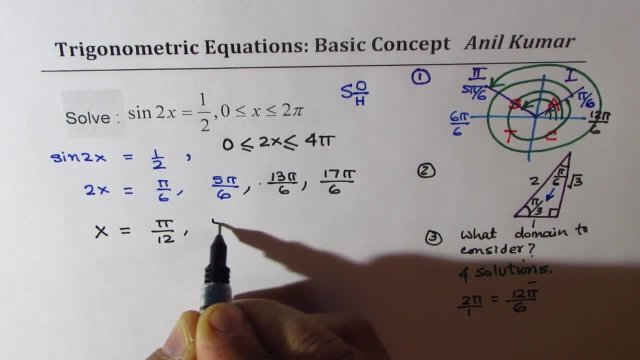 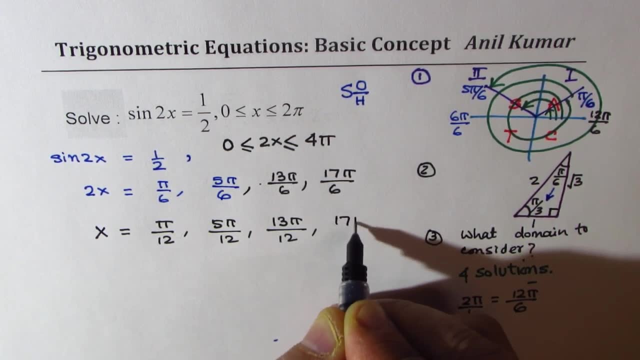 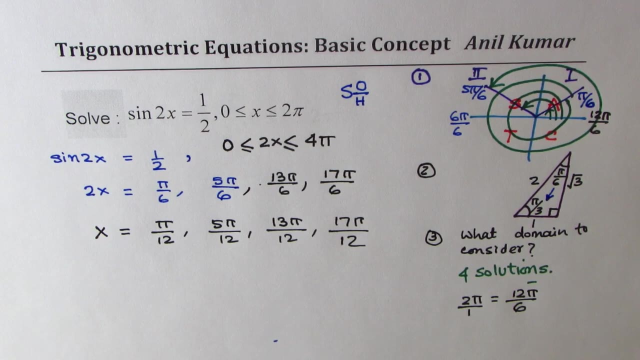 So we get pi by 12, 5 pi by 12, 13, pi by 12 and 17 pi by 12 as four answers. So we have four solutions to this particular question. I hope that concept is clear, right. 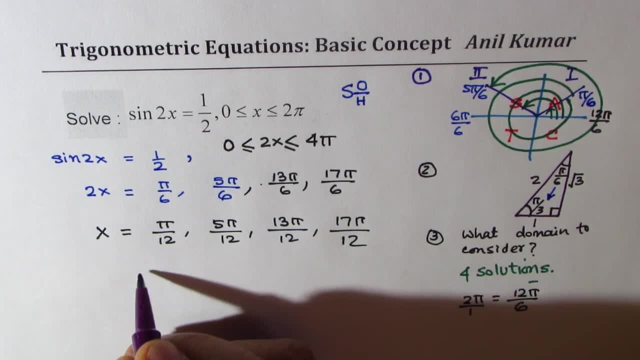 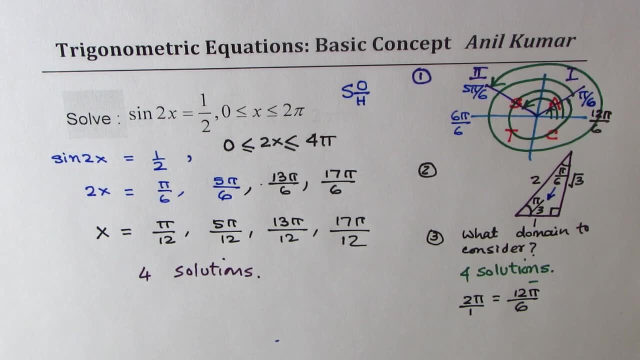 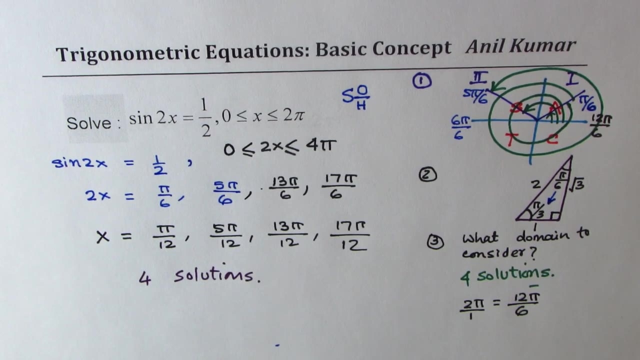 So note for this. we have, as expected, four solutions. Perfect, now I will change this question from sine to cosine and let us see if you could do it. So let us move on and take our practice question. Now here is a question for you to practice. 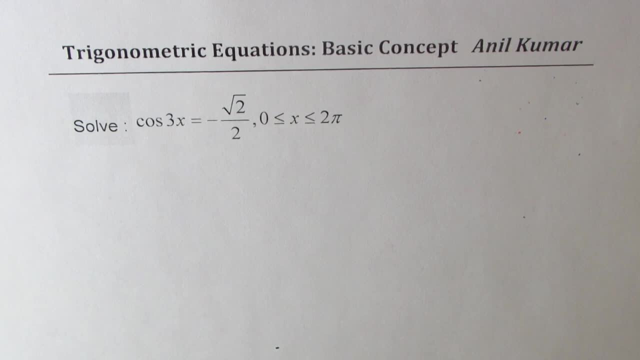 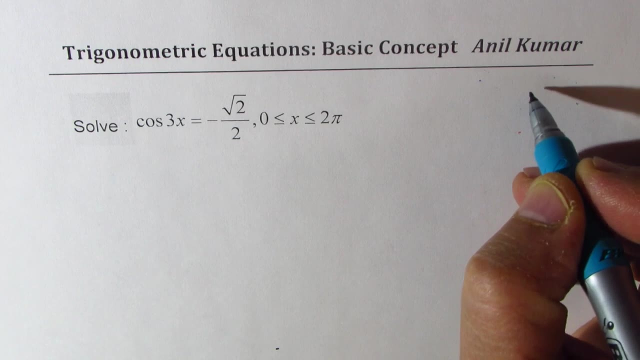 You need to solve: cos 3x equals to minus square root 2 over 2, where again x is between 0 to 2 pi. So how are you going to solve? Let us look into our strategy. What are we expecting? 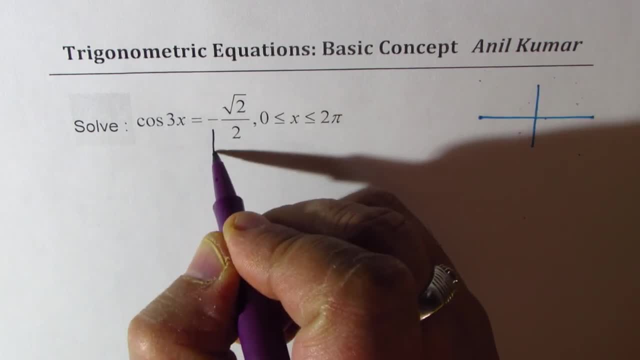 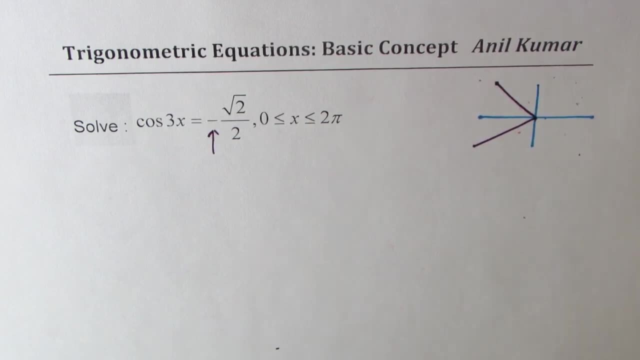 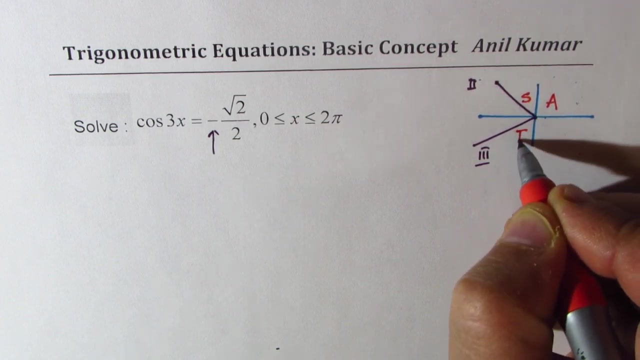 Well, cos negative, right, You see this negative part. So cos is negative in these two quadrants? Perfect. So we are expecting solution in quadrant 2 and in quadrant 3 this time, Since we know that all are positive here. sine is positive in quadrant 2, tan in 3 and 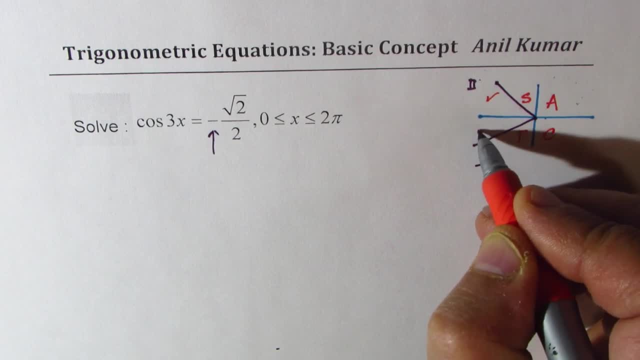 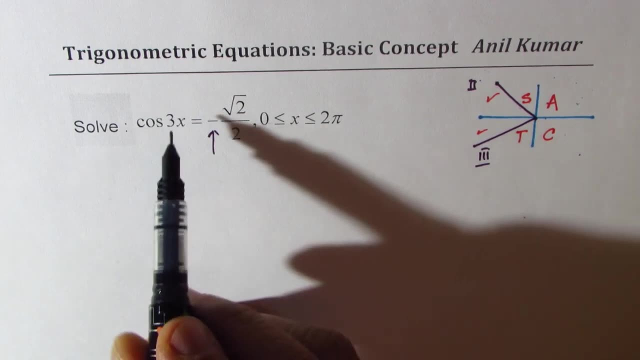 cosine in 4.. So cos is negative in quadrant 2 and 3.. Perfect, That is first part. And then we also note that we are talking about 3x. We are given x between 0 and 2 pi. 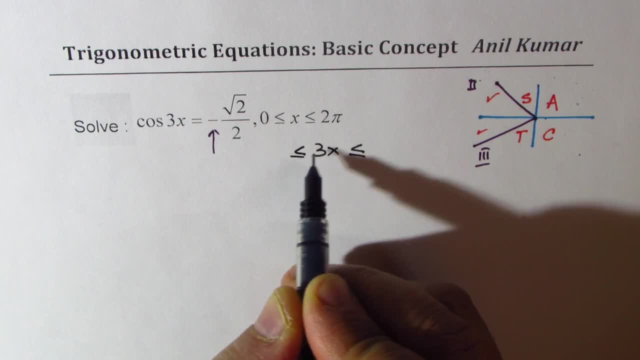 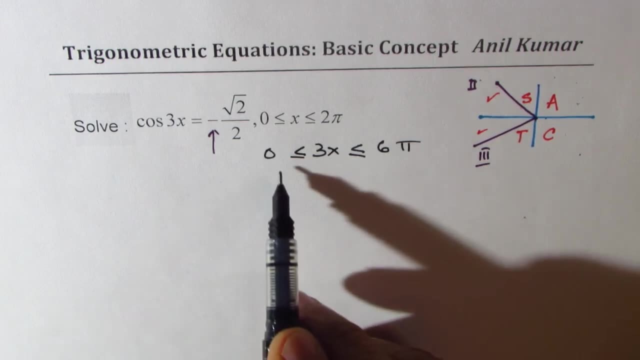 So what will happen to 3x? We have to multiply this by 3.. 3x will be between 0 to 6 pi. Do you see that 0 to 6 pi means we have how many solutions? 2 in 2 pi. 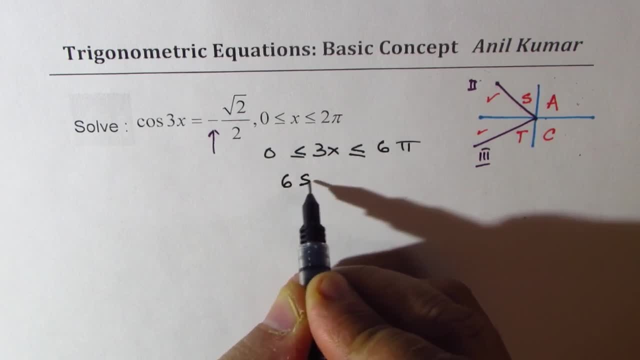 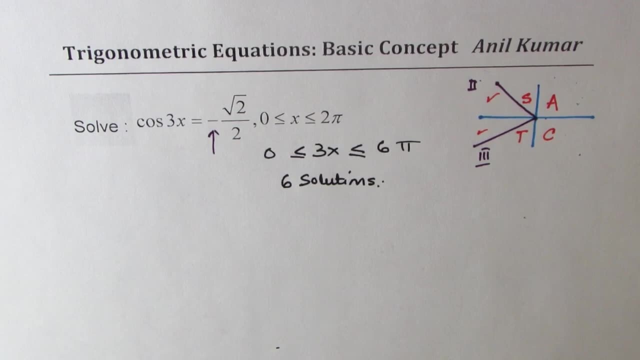 Then in 6 pi, So we are expecting 6 solutions. Do you get the idea Right? So we are expecting 6 solutions. Now, which is the special triangle we are looking for. Square root 2 over 2 reminds you of pi by 4, right? 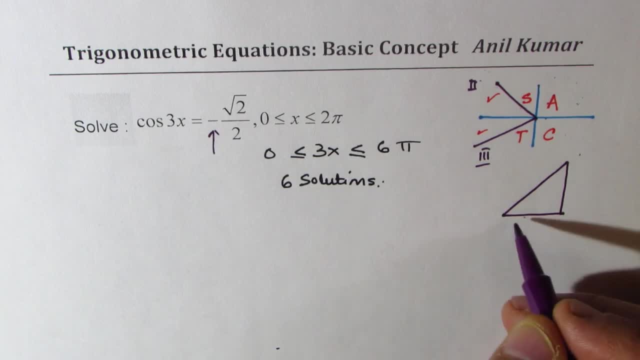 So that is the triangle we are looking for, Perfect. So if each side is square, root, 2. …. 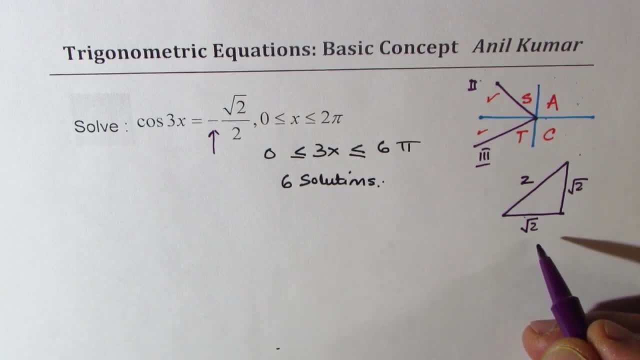 2 over 2.. Then the hypotenuse is 2 square root 2.. 2. This square plus this square square root, and the angle here is pi by 4.. Perfect Now when you are adding pi by 4, right when you are counting in terms of pi by 4,. 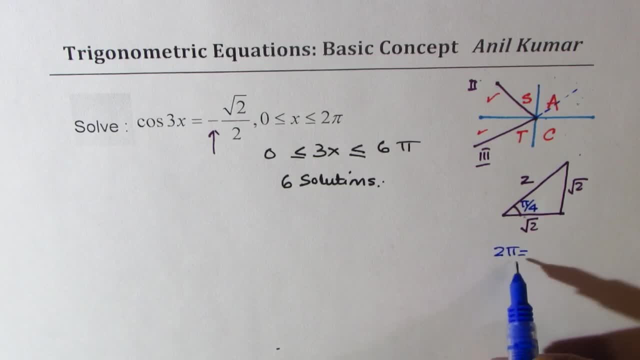 in that case 2 pi could be written as 8 pi by 4.. So we will add 8 pi by 4 to our solutions to get six solutions, starting from the first two. You get the idea Perfect. So let us begin. 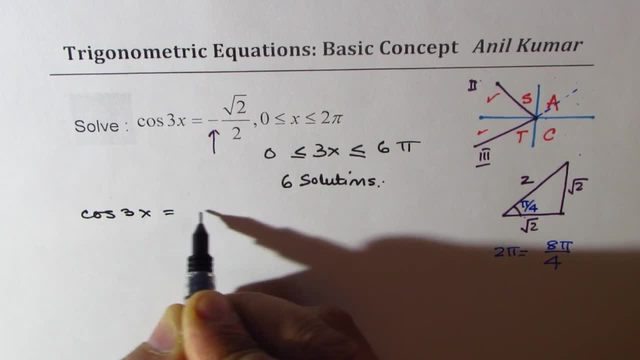 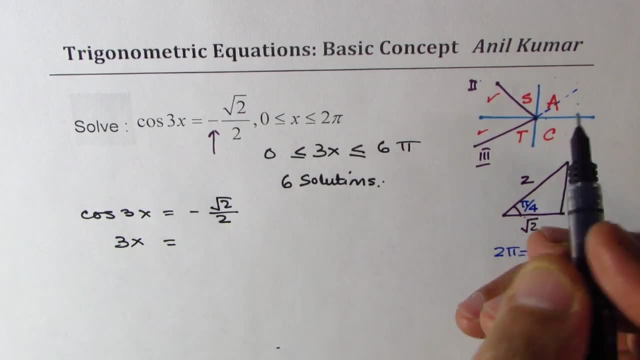 So we have: cos 3x equals to minus square root 2 over 2.. Now that means that 3x should be equal to. we are looking for solutions in quadrant 2 and 3, each angle is pi by 4, right, So for pi. 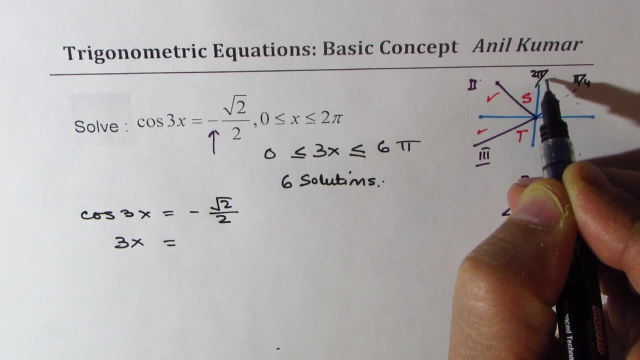 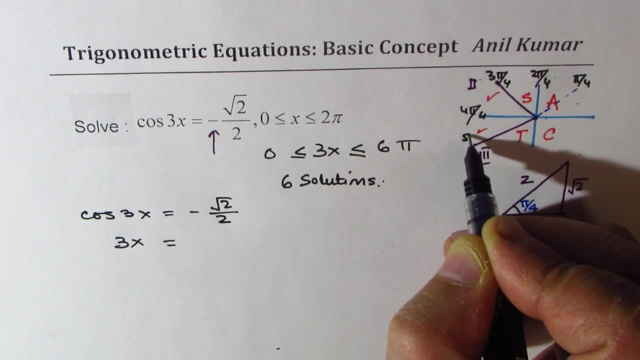 by 4, this is pi by 4, this is 2 pi by 4.. 3 pi by 4.. This is 4 pi by 4.. This is 5 pi by 4.. So the two solutions are 3 pi by 4.. 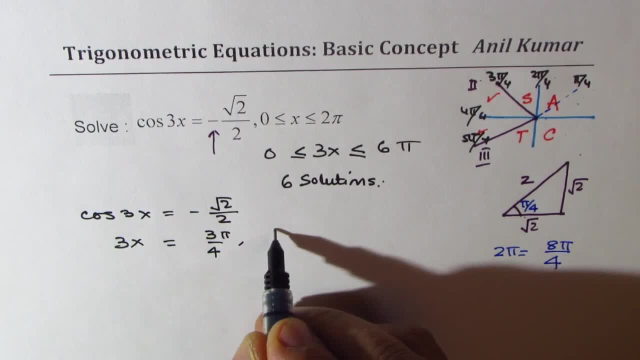 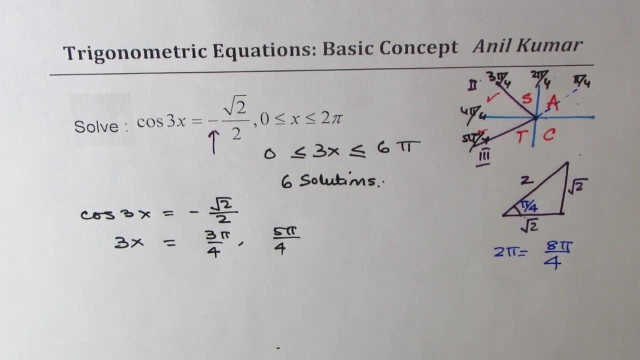 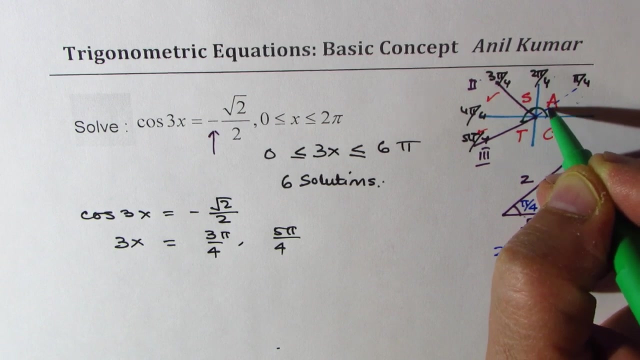 This is in quadrant 2, and 5 pi by 4, which is in quadrant 3.. Now we have to go two more circles, right? So we got a solution which is here and then there, But we need to go. 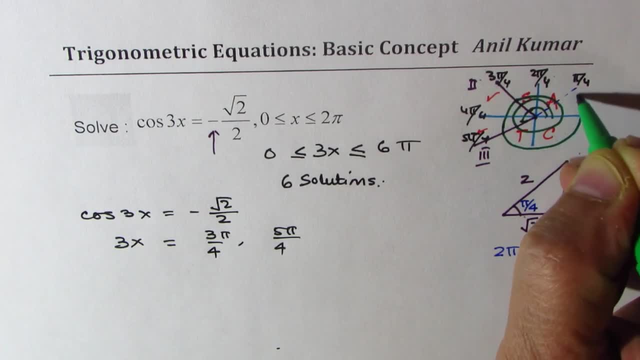 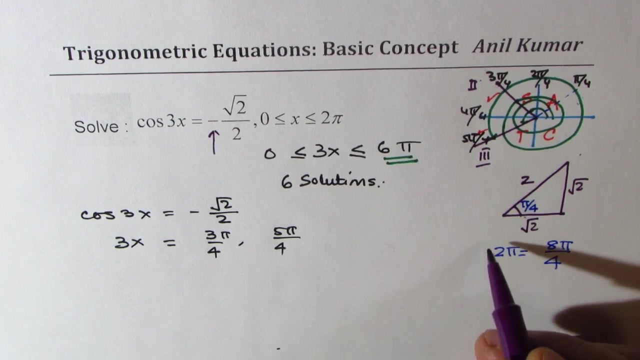 full circle, come back to these points and then again go full circle and come back to these points to get all the six solutions. That is to say, we need to add 8 pi by 4. now, Perfect. So this is what we are going to add to our solutions. 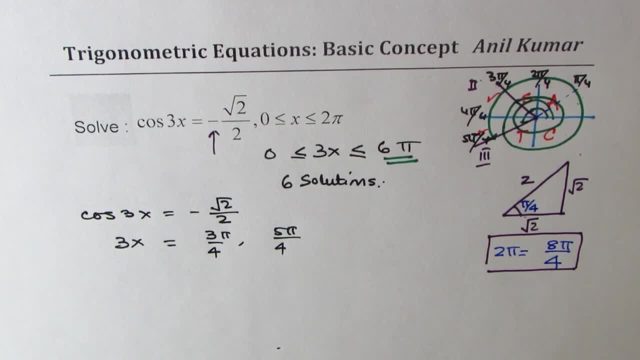 To get other four solutions. So 8 plus 3, 8 plus 3 is 11.. We get 11 pi by 4.. 8 plus 5 is 13.. Then again we will add 8. So we get 19 pi by 4 and 8 plus 13 as 21 pi by 4.. 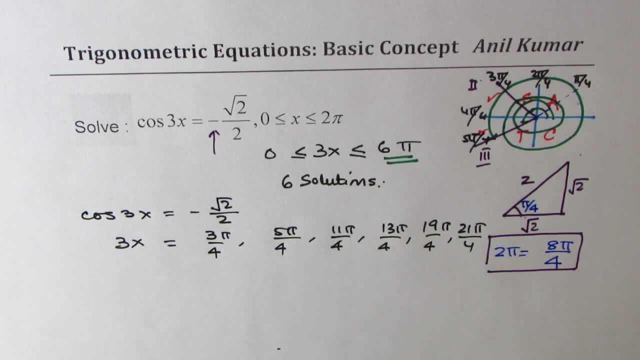 Do you see that part? So that is how we are going to get our solutions. Now, x is what, This is 3x. So the answer is: x is equal to. we are going to divide them by 3 now. 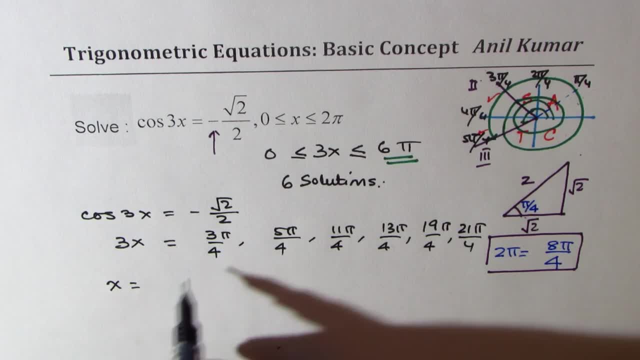 correct. So dividing 3 by 3 is 1.. So we get pi by 4 for the first one Here, 5 pi by 12, then 11 by 12,, 13 pi by 12,, 12.. 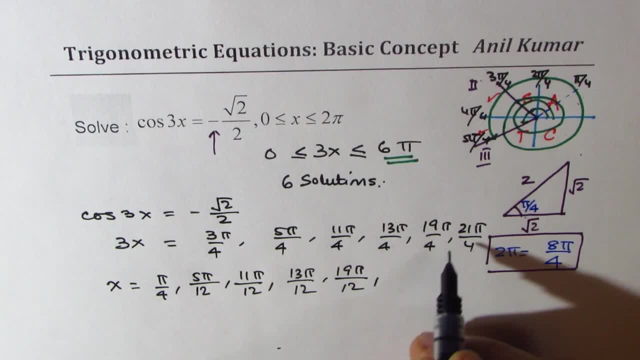 19 pi by 12 and 21 could be divided by 3, 7, right? so we could write this as 7 pi by 4.. Do you see that part? So that is how you get 1,, 2,, 3,, 4,, 5, 6 solutions, and that becomes the solution set for the. 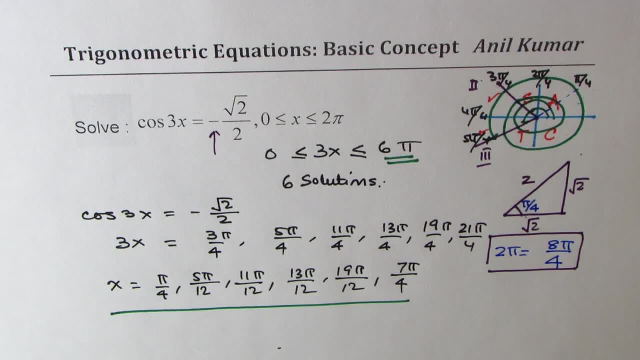 given equation. So I hope the concept is clear. So remember one thing, that is, whenever we need to solve in a particular domain any trigonometric equation, we should actually modify the domain as per the question, right? So modify domain and find all possible solutions.